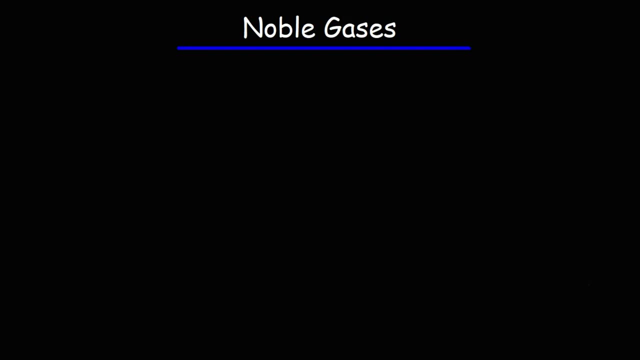 In this video we're going to talk about the noble gases. The noble gases are found on the right side of the periodic table and it includes gases like helium, neon, argon, krypton, xenon and radon. The gases are found in group 8a or group 18, of the periodic table. Now, these gases are fairly non-reactive. They're chemically inert for the most part. 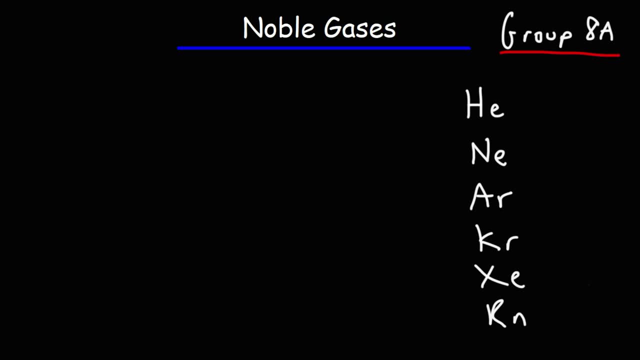 Some of them, however, can participate in reactions like krypton and xenon. They can form stable compounds with very reactive elements like fluorine, and we'll talk more about that later, But for the most part they're non-reactive. 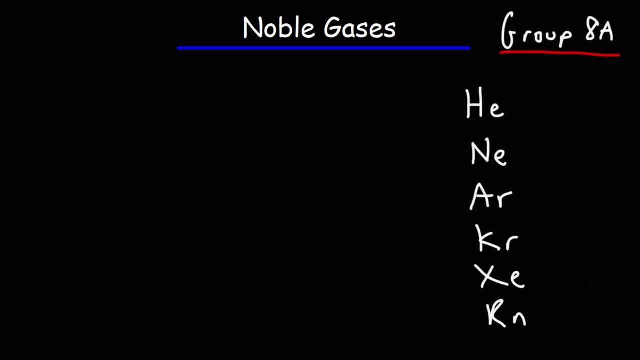 When they're chemically inert they don't really want to react. They're fairly stable, And this is because their outer energy levels are filled with electrons. Helium has two valence electrons, Neon has eight valence electrons, Argon, krypton, the rest. they also have eight valence electrons as well. 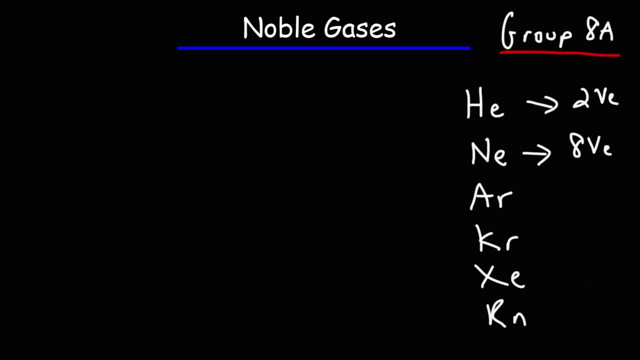 But their outer most energy level is filled with electrons, And that explains the unusual stability that this group of elements have. Now, as you go down a group, the boiling point of the noble gases increases. The atomic radius increases as well. Helium has a boiling point of around negative 270.. And this is in Celsius. For neon it's negative 246.. Argon negative 186.. Krypton is negative 153.. Xenon negative 107.. And radon negative 62.. 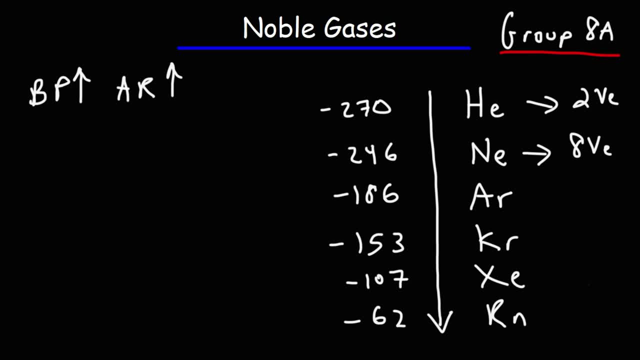 So those are the boiling points of the gases. As you go down, as the atom becomes bigger, as the atoms gain more electrons, their boiling point goes up. The only forces acting on these atoms are LDF, London Dispersion Forces. 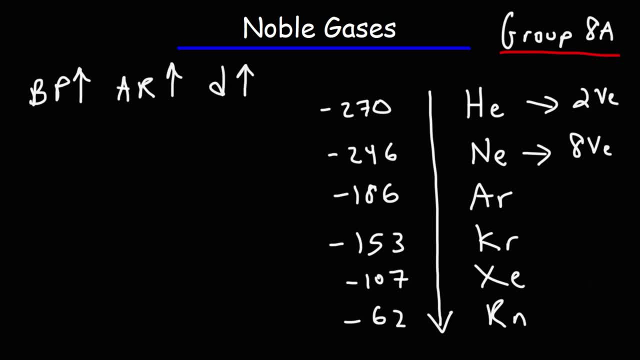 Now, as you go down a group, the density of these atoms increases as well. Xenon has a higher density than neon. Now these elements are monoatomic. They exist as single atoms. So helium is monoatomic. We don't have diatomic helium. 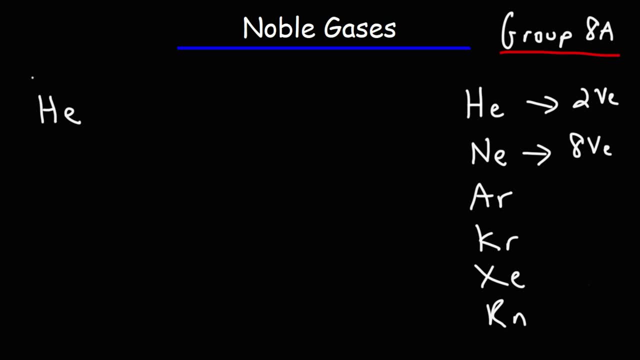 Helium exists just as a single atom, The halogens, for instance. they are diatomic. So elements like fluorine, chlorine, bromine, iodine, all of these halogens, they're diatomic, They're molecules composed of two atoms. 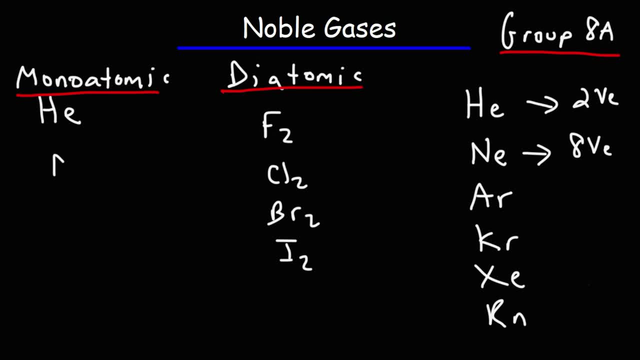 Whereas the noble gases, they're monoatomic. They're composed of just atoms instead of molecules. Ozone, which is an allotribe of oxygen, This is oxygen gas. Ozone is a molecule with three atoms. I guess you could say it's triatomic. 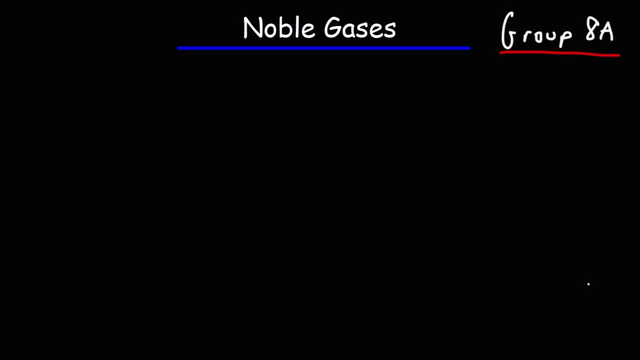 Now let's talk about some of the reactions. Let's talk about some of the reactions of noble gases. Xenon gas can react with fluorine. Xenon doesn't react with most elements, but fluorine is extremely reactive. It's one of the most reactive elements out there. 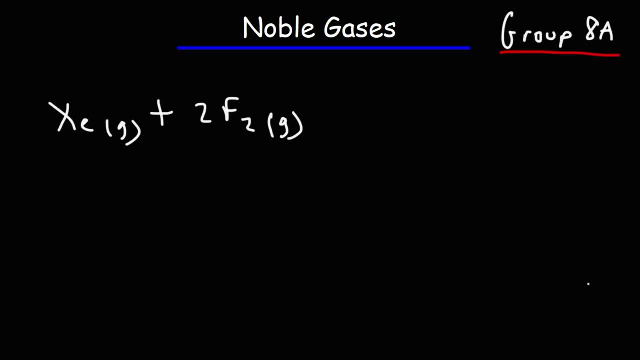 It's strong enough to react with the stable xenon gas And it can produce this compound, Xenon tetrafluoride, which is a solid. It can also produce other compounds like xenon hexafluoride. Xenon hexafluoride can react with water. 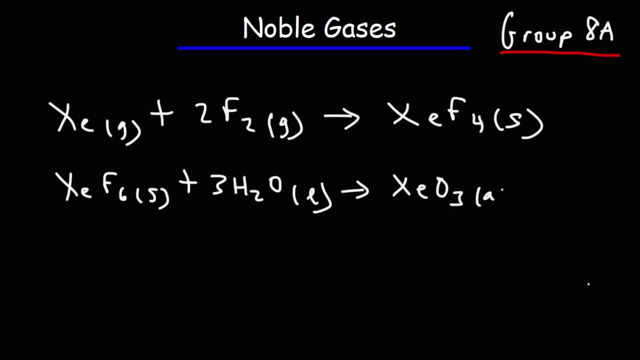 to produce xenon trioxide and hydrofluoric acid. Krypton can also react with fluorine To make this compound, Krypton, difluoride. So the noble gases. for the most part they're not truly inert. 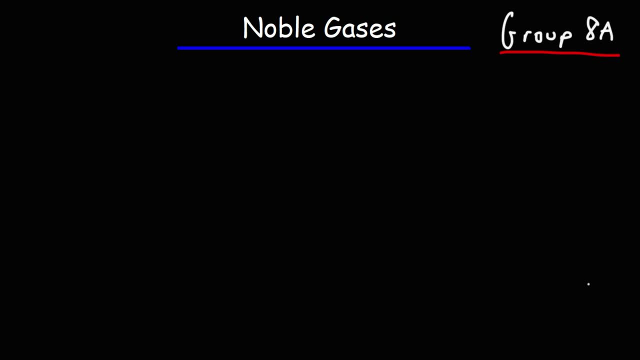 They can react, But not all of them react, though For the most part they're fairly unreactive. It takes a very reactive compound, I mean a very reactive molecule like fluorine, to get them to participate in chemical reactions. 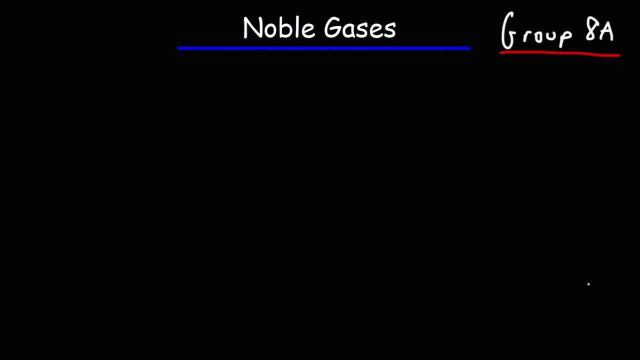 Now let's talk about some of the properties of the noble gases. Helium: You've seen it in helium balloons. Helium is lighter than air, So when you fill up a balloon with helium, those are the balloons that will rise.